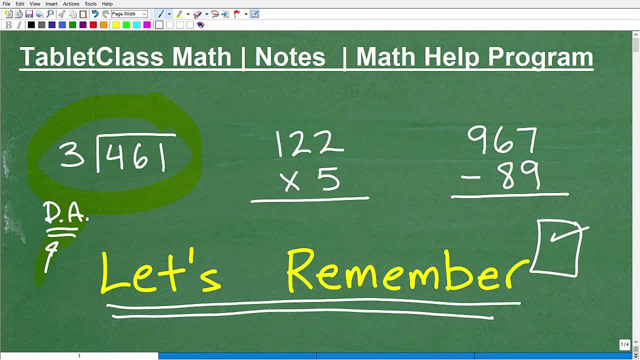 Okay. so again, it's all kind of ties in. But you know, it's understandable that our arithmetic skills would decrease over time, right, Because there's that dependency on calculars. But I went to elementary school way back in the 1970s. That was awesome time. I grew up in Southern California And it was definitely a different time. error, because I remember my first grade teacher smoking in the classroom. 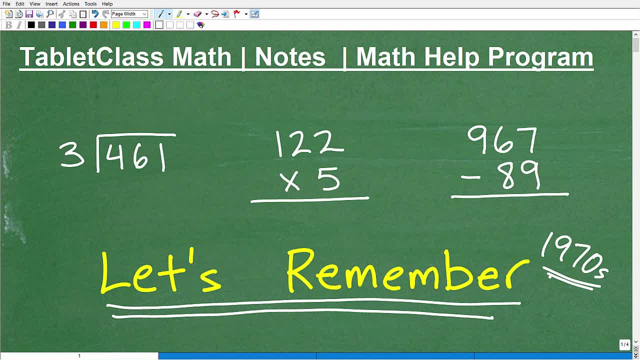 She was probably saying: these kids they're, they're just, you know, they're driving me crazy, And anyways, it was. it was. we probably were driving her crazy as well, But it was an awesome time to go to school, at least in my memory. I mean, we had our recess time. I could still remember that today, And that's what I don't know- 40 years ago, maybe even longer than that. But the bottom line is this: you know, I thank my teachers because I still remember this arithmetic, Okay, because we did a lot of it, especially. 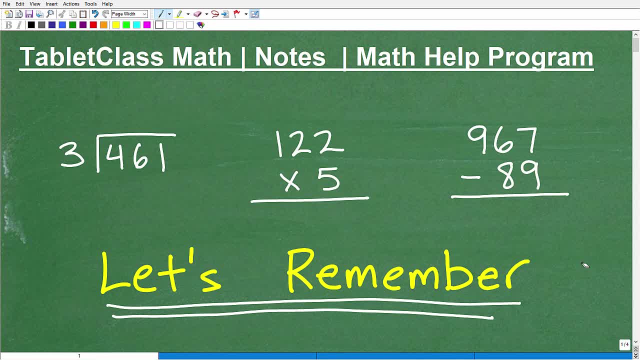 back in those days because you know we really didn't depend on calculars. But the bottom line is this: no matter where you're at in your education, you need to know and remember your arithmetic. Now I will say this: much: Arithmetic is being taught in a couple different stylistic ways or different approach, depending on what kind of curriculum you're using, And a lot of people don't have good feelings about common core. whatever your stand is on that, The bottom line is this: you 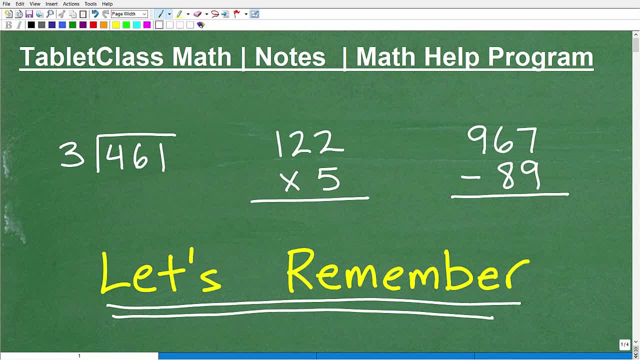 need to be able to get the answers on this. So if you've learned arithmetic- you know, if you're kind of a recent student and you learned it in a different way- well, I'm going to go through how to do these particular problems in a more kind of traditional old school way, But the bottom line is that you need to be able to get these answers right. right, So we're just going to look at three simple examples. All right, we're going to do this division problem, we're going to do this multiplication problem and we're going to do this subtraction problem. I left addition out because I thought subtraction would be more interesting. 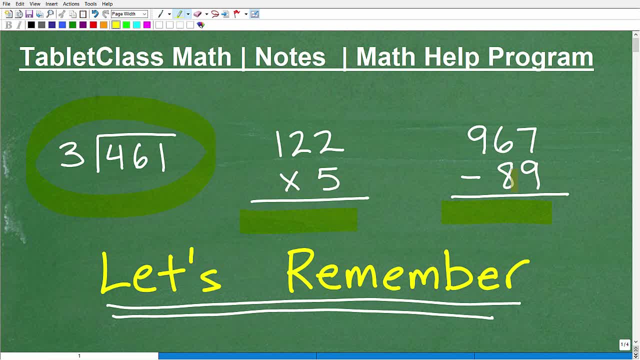 Now, of course, before we start doing this, I'd rather have you challenge yourself. just pause the video real quick. You know these prompts should take you no more than 60 seconds to do. knock them out real quick, see where you're at right. But you know, the main point of this video is not: hey, we're going to do three little prompts here. The main point is to emphasize where arithmetic is important in mathematics. it's important that you know this stuff. There's gonna be plenty of times where you'll have exams where you are not able to use a calculator. 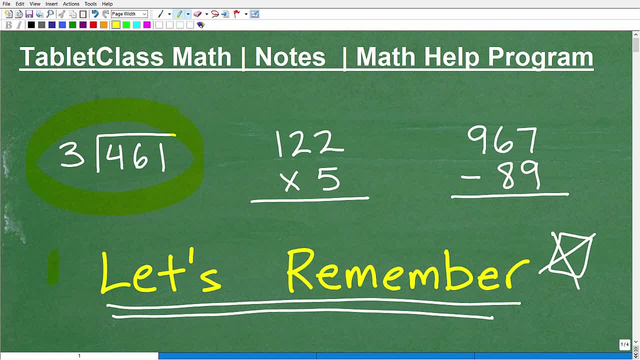 And even division. okay, as you progress in your mathematics- Now I don't know if you are in algebra or taking algebra two or any more advanced course, But we use this to do this problem. we use something called the division algorithm. Okay, now most of you are like: I don't really care what it's called, I just know the steps to do it. Well, listen, the division algorithm. we need to know this algorithm because this is very important. 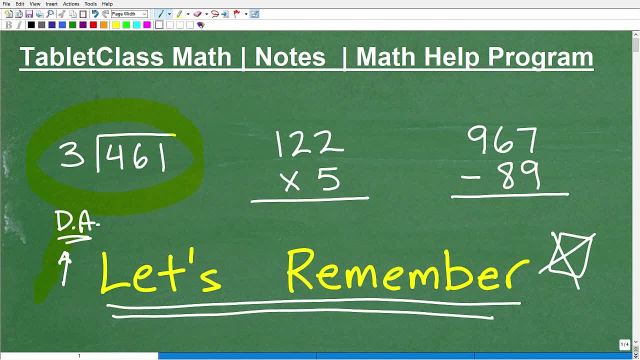 When we're dividing polynomials, long division, etc. So again, just believe me when I tell you you got to know your arithmetic And it's, you know, hopefully, kind of like riding a bike. Once you start doing this stuff again you'll be like, okay, now remember how to do it right. You just will hopefully come back to you. So you know, we're going to look at these three problems. Of course I'm going to do them step by step here And just one second. but this won't be fun, Unless you try them yourself, of course, without the aid of a calculator. 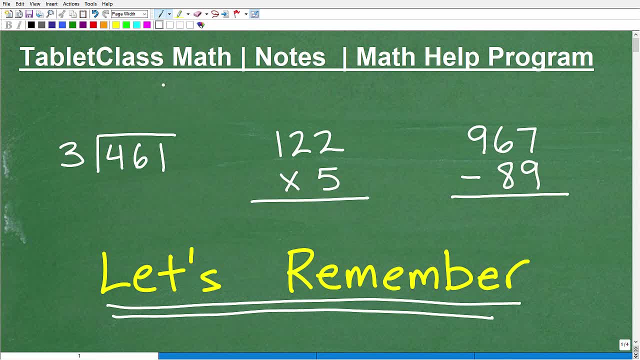 But we'll get to these problems in just one second. But first let me quickly introduce myself. My name is John. I'm the founder of Tablet Class Math. I'm also a middle and high school math teacher And over several years I've constructed what I like to believe is one of the best online math help programs there is. Of course, I'll let you be the judge of that. If you're interested, you could check out my math help program by following the link in the description of this video. But basically I have 100 plus different math courses, ranging from pre-algebra, algebra one, geometry, algebra two I'm going to be launching next week. 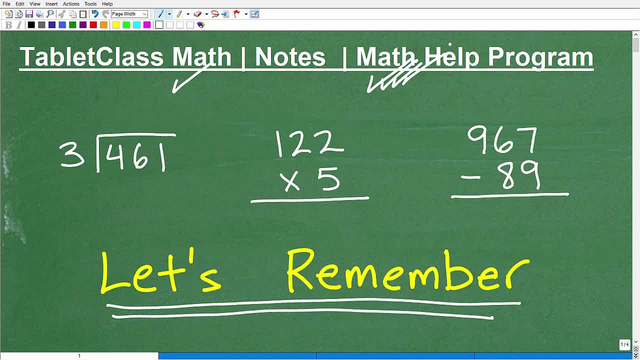 Pre-calculus here shortly, But I also do a lot in the area of test preparation. So if you're studying for the GED, SAT, ACT, GRE, GMAT, ASVAB, Accuplacer, CLEP exam, Alex exam, teacher certification exam- any number of exams- let me help you prepare. Just go to my website and check out my full course catalog. If I do not have the exam you're studying for, drop me a line and I'll help you out the best I can. I also do a lot with independent learners, like homeschoolers, So if you 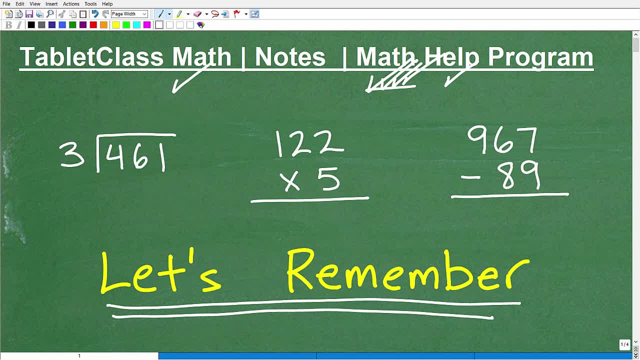 homeschool. I've been working with homeschoolers for 15 plus years. I have a great homeschool learning system, So you might want to check that out And then, obviously, help those of you that are just struggling in your math courses. Now, if you are truly serious about wanting to learn math, then you have to be serious about this. Okay, over decades of teaching math, it's apparent to me those students who work hard okay, take great math notes. they always they end up with like excellent grades almost all the time right, And the reverse is true. Those students who like to 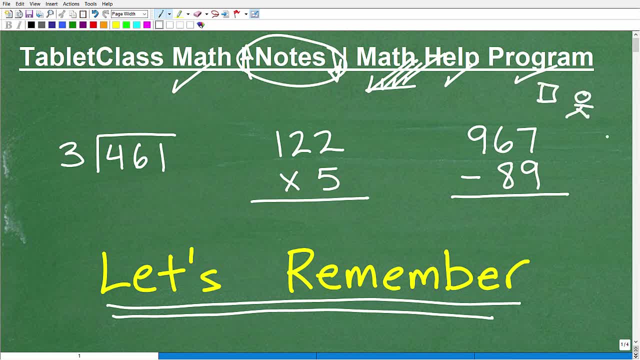 check out their cell phone, talk to their buddies in class and, you know, pretend that they're taking notes, But really, in actuality, what are they doing? They're doing their homework for another class. Listen, I did all these things, these things, way back in the good old 1980s, except. 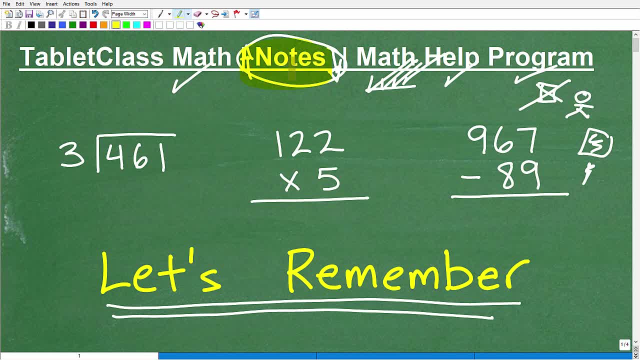 for the cell phone part. we didn't have cell phones. But listen, if you want to be successful in anything, you've got to focus and put in the work, And when it comes to math, that means taking excellent notes. But as you're improving, you still need something to study from, because you probably 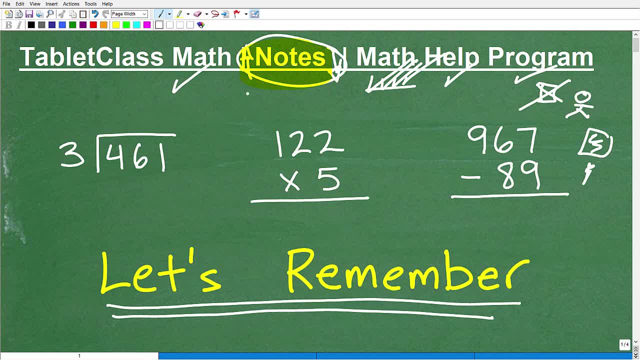 don't have notes from the previous materials, So I offer detailed, comprehensive math notes to include pre-algebra, algebra 1, geometry, algebra 2, trigonometry. You can find the links to those notes in the description of this video. All right, so here's our three problems. Again, I'm going to 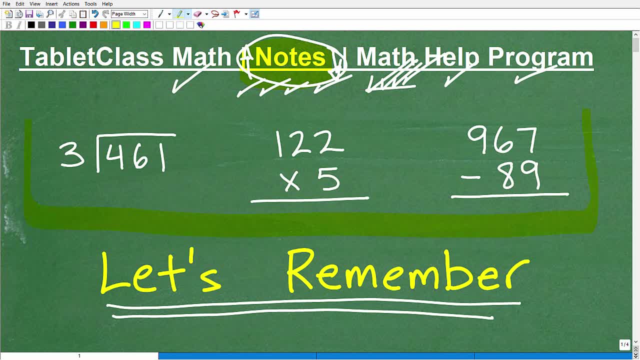 do this in a kind of old school way, the way I was taught. Now, the way I'm going to do these steps- okay, may not be the exact way that you're going to do them, but it doesn't make a difference, as. 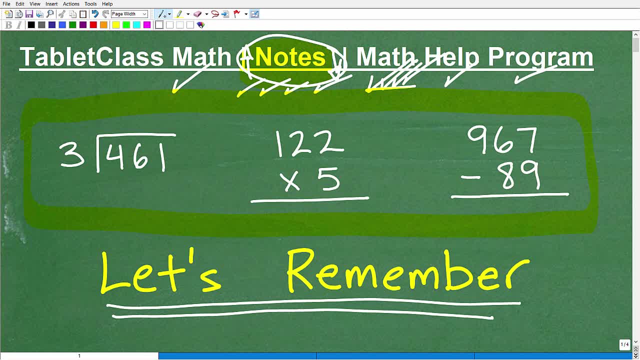 long as you get the answer right is what counts, Because there is a little stylistic, different ways, formats and stuff that you could be taught. Now, if you're going to do this in a completely different way, you know long as the way you were taught and you can get the right. 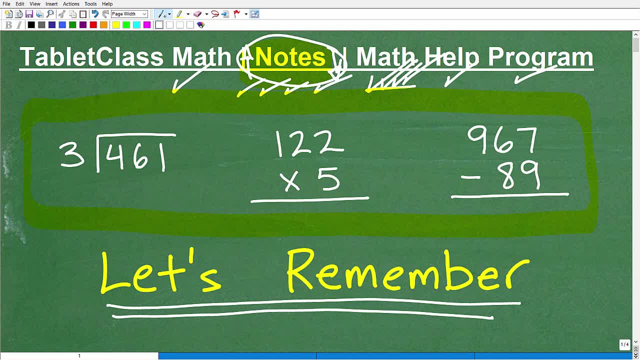 answer again. that's what counts. All right, but I'm going to do it the way I was taught way back in the good old 1970s in Southern California. All right, so let's get to it, And maybe we go to my. 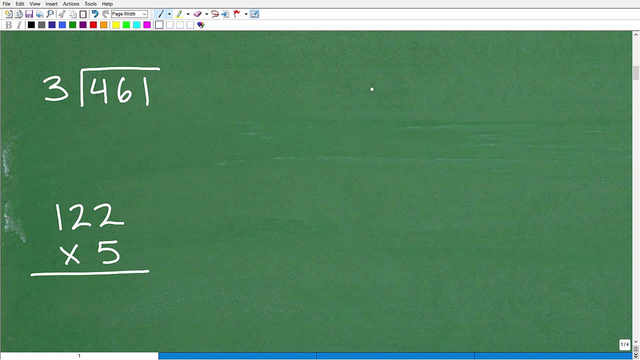 first problem. Let's just start off with this division problem. And here we go, Right, so I'm division here. that's a whole nother deal for 61.. All right, so we're gonna take 461, I'm going to. 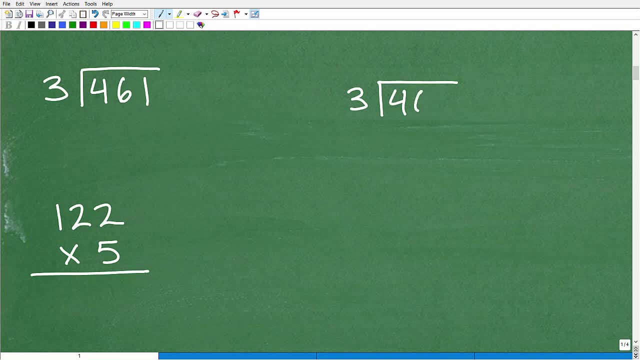 divide it by three. Let me draw that a little bit better. So what do we do? Well, I'm going to be like, okay, three, I'm going to look at this first number. Can three go in that first number? Yes, 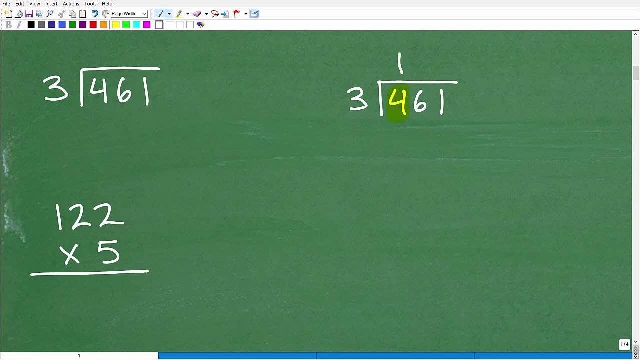 it goes into it. what one time. So I'm doing right now what we call the division algorithm. right, Three goes into four, one. then I have my answer. I'm going to put it over this four spot right, I'm going to go one times three. 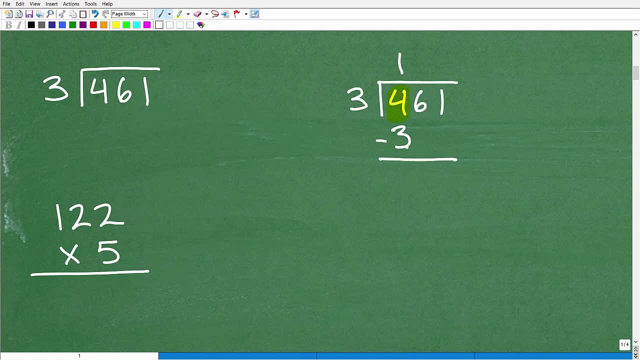 That's three. Okay, then what I do now? I'm going to subtract right, then I'm going to go, or three, take away four, or four minus three, that is one, Okay, so that's like the first step. I'm like 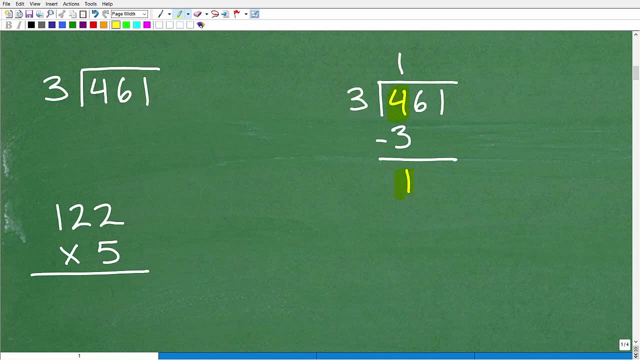 all. right now I'm going to ask, ask myself: can three go into this one? No, I cannot. So what do I do? I need to drop down that six, that next digit. Okay, so I bring down that six. Now I'm. 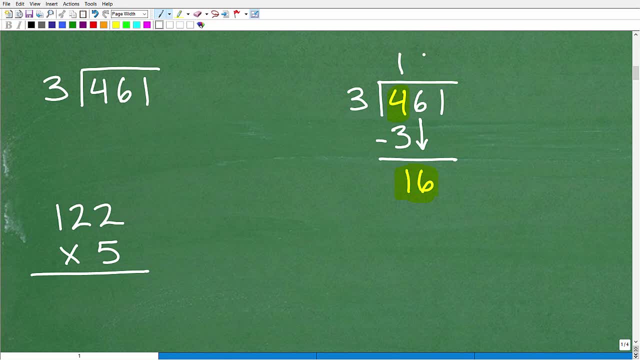 going to ask myself: can three go into 16?? Oh, indeed it can. three goes in 16.. Five times. So I'll put a five there And then I'm going to repeat the process. I'm going to go five times. three is 15.. 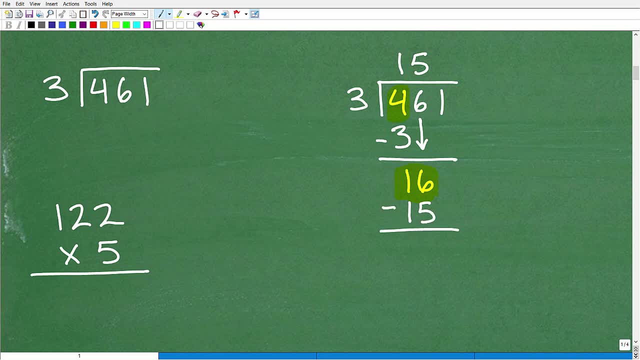 And then I'm going to go ahead and subtract, right, So hopefully this is kind of like: oh yeah, I remember this. All right, I get a one right there, Okay. then I'm going to ask myself again: can three go into one? No, it cannot, Right, Three cannot go into one. So I'm going to 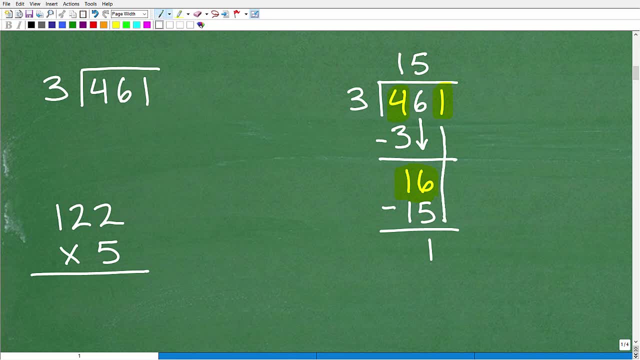 take that one. I'm going to drop it way down Over here, right there. Okay, So can three go into 11? Yes, it can. How many times? Well, three times three is nine. three times four is 12.. So it's going to be three. So three times three. 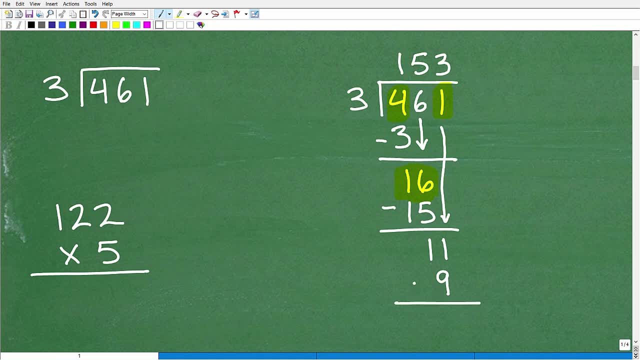 is nine. Okay, and now I'm going to go ahead and take away subtract. there I have two And I can three go into two. No, Hey, but there's no more numbers to drop down, So you are done. So the 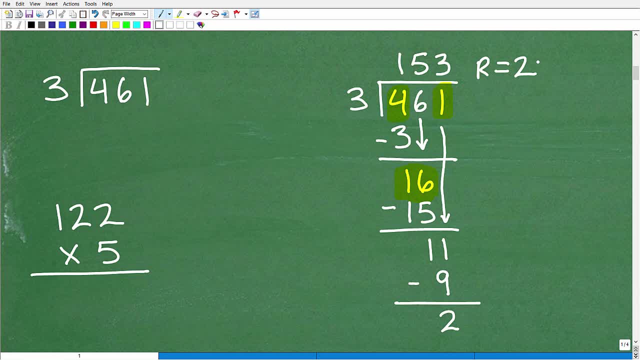 remainder two. Okay, now of course you can put that as two thirds, But this is the answer, And if you got that right, I will have to give you a little happy face and a checkmark and we'll give you like three stars. I don't know if you remember way back in the good old days, elementary. 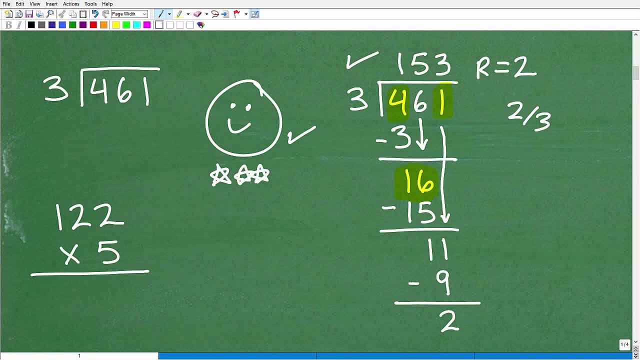 school. I remember this is probably like 1976. The teacher giving you a bunch of stars and you know for you know being on time and doing all the things you're supposed to be doing. It was a great feeling. 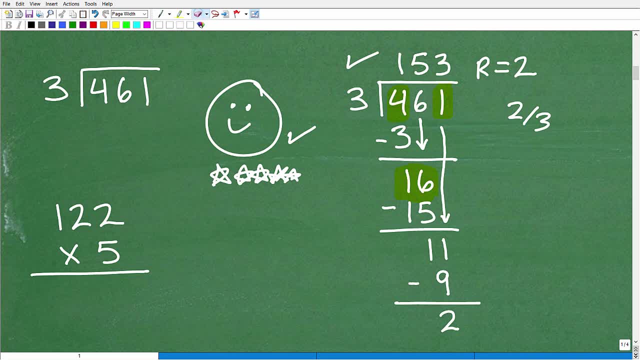 So if you got this right, good stuff right. So that's the first problem, And now let's move on to our second problem. All right, now our second problem is multiplication. And now these are very easy problems. I don't want to, you know, you know, do like triple digit, you know like four. 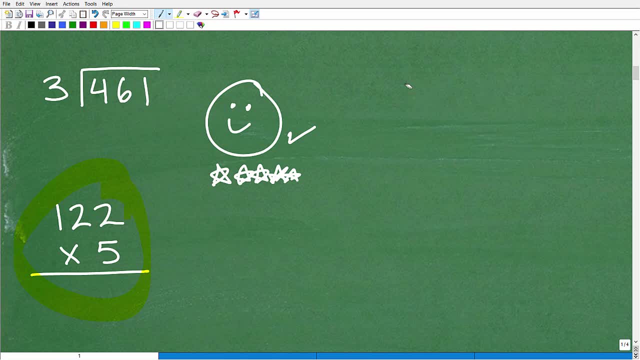 digit number times the three digits. it takes you long, So let's just go ahead and do this one here. 122 times five, okay, so what do we do, All right? well, again, some of you might have learned this a little bit. 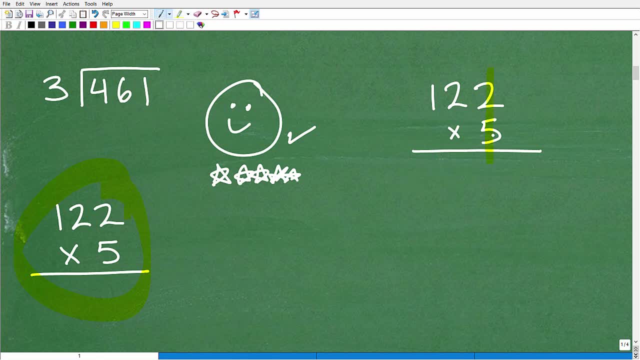 different way. But first thing is, you got to multiply these numbers. So five times two is 10.. Okay, great. Or do I put 10 right here? No, you do not put 10.. What we're going to do is going to put. 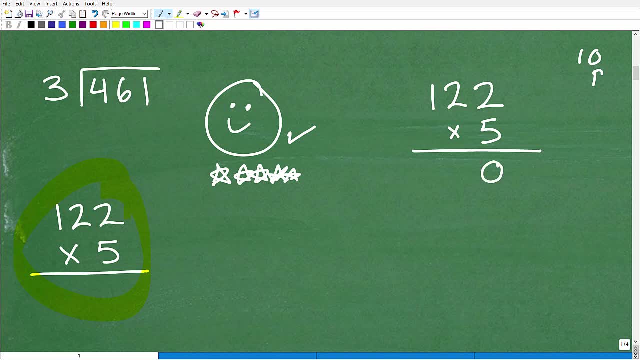 that digit zero right there. right, Then I'm going to carry the one. So this one and zero is my 10.. All right, that's the answer Now. okay, I just did this. I'm going to multiply this way again. So five times two is 10.. But now I'm going to add this little one, because I carried 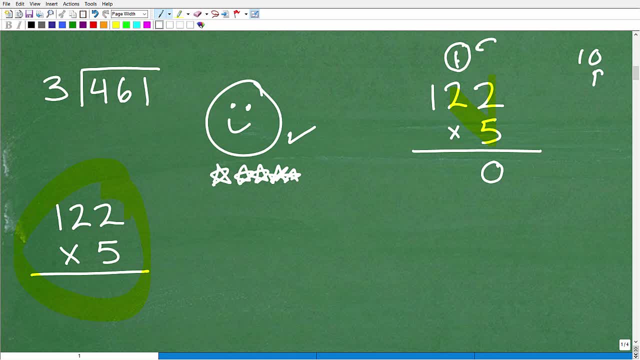 this one over. Okay, so so 10 plus one is what, that's 11.. So I'm going to put this digit right there And I got to carry that one again, So five. I'm going to go ahead and continue the process. 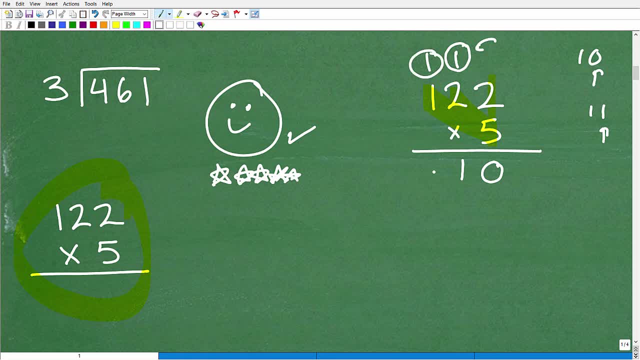 five times one is five. I'm going to add that one that's six, So that's 610.. That is the final answer. Okay, So if you got that right, let's give you another checkmark And we'll throw in a couple more stars for good order. All right, All right. 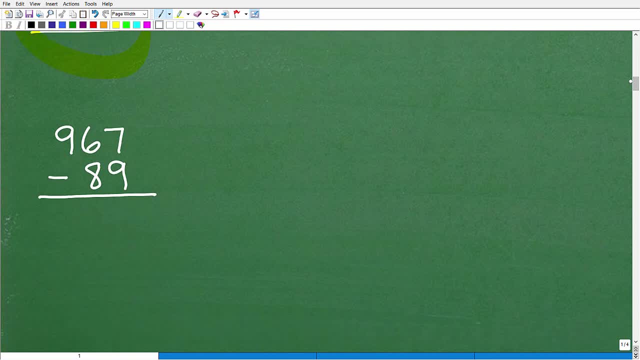 let's go ahead and finish up with our last problem. So I got 967.. And I'm going to subtract 89 from that number. Okay, All right. So what do I do? Well, this is not addition, this is subtraction. Okay, So first thing is I'm going to focus on this column. 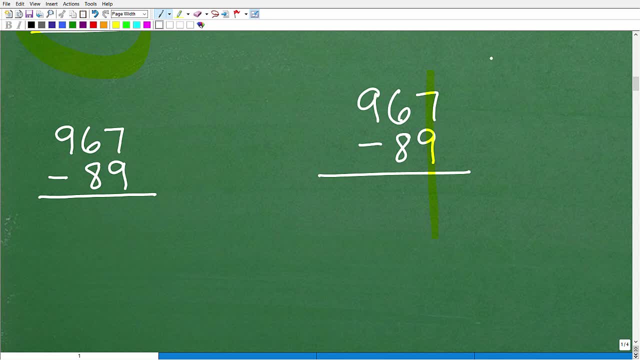 Now can I take nine away from seven? No, if I have. let's just look at here: one, two, three, four, five, six, seven. I have seven items here right: One, two, three, four, five, six, seven items right here. Can I take nine items? 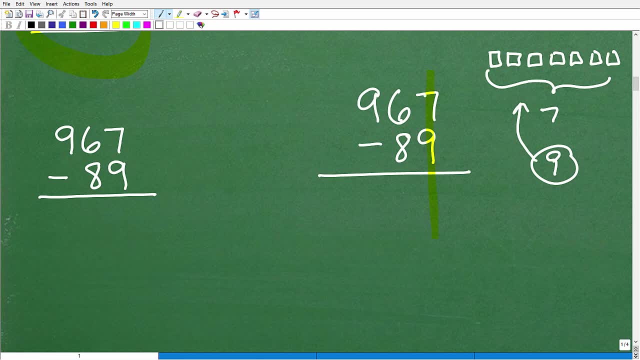 away from those seven items? No, I cannot. We're not dealing with like positive negative numbers here. Like what do I do here? I can't take nine away from seven. There's not enough things to take Nine, I need at least nine things to take nine away. So I'm confused. Well, what we need to do? 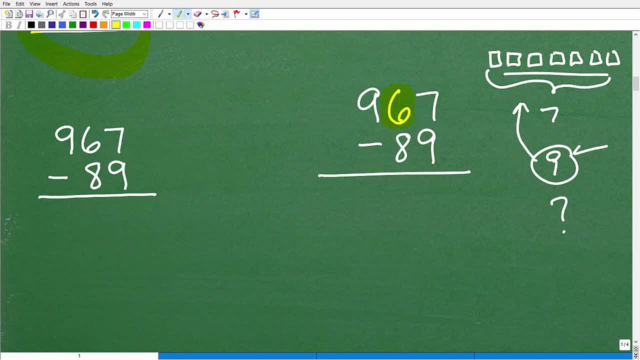 is borrow. Okay. So this little six right here, we're going to borrow some numbers from it with some digits. Okay, We're going to like: all right, six, I'm going to make you into a five And I'm going to put a one right there. Okay, Now again how you learn this, or the format. 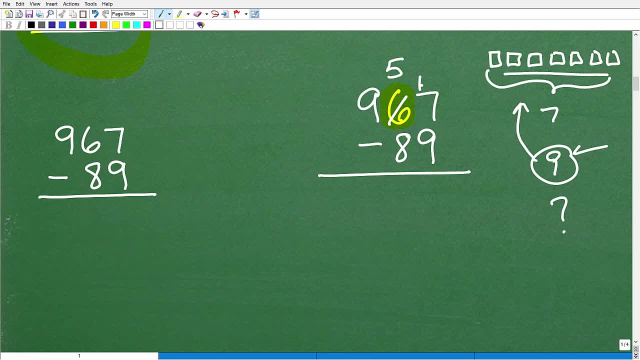 that you're using. as long as you get the right answer, that's all I care about. So now I have a seven That's a one, and seven That's a 17.. Now can I take nine away from 17?? Absolutely, Yeah. 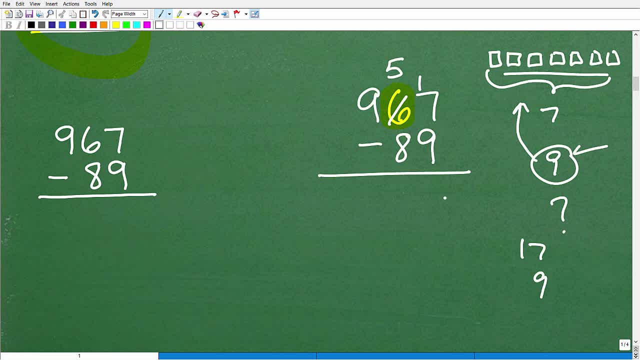 What's my answer there? Well, I believe that answer is going to be eight, Okay, All right, So nine, take away nine from 17 is eight, Okay. So now I'm good here. So now I'm going to bring my. 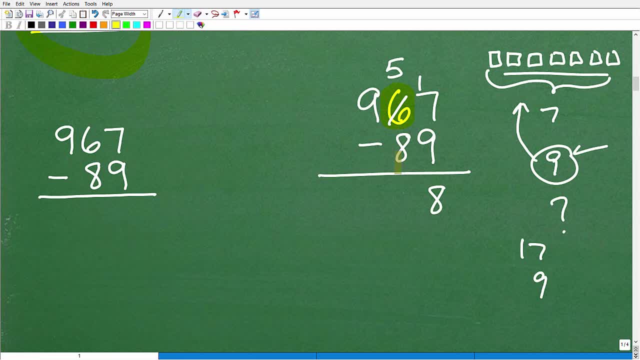 attention to the second column. So I'm asking myself: can I take eight from five? No, I can't. It's like this situation: I don't have enough items. I can't take nine away from 17.. I can't take. 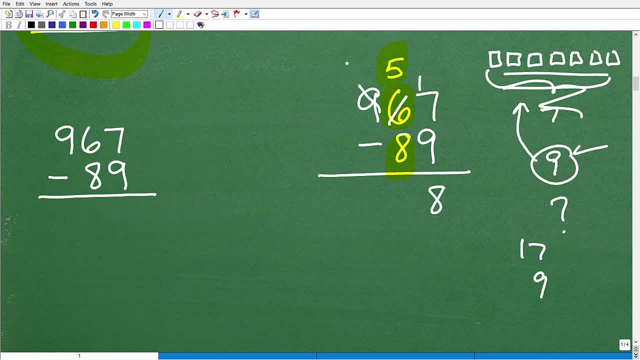 numbers here, So I'm going to have to borrow again across that nine. Now I'm going to make that into an eight and I'll keep that as a 15.. Okay, So can I take away eight from 15? Yes, I can. All right, So what's that answer? That will be seven. Okay So, eight take away or 15 minus. 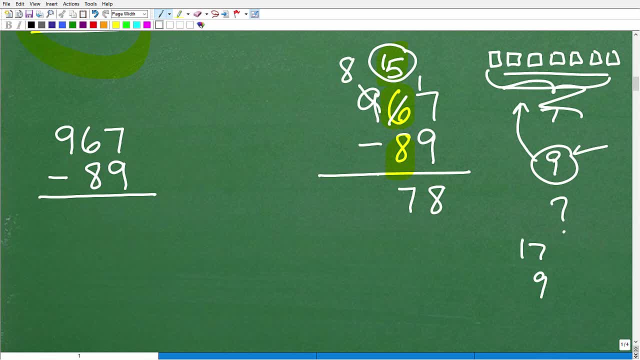 eight is seven. Now, what's left here? I just have nothing left, All right, Cause I already did my little subtraction with these two digits, So that little eight is just going to plop right down here. So my answer is eight, 78, and that is it. Okay, So if you got, uh, the all three of these, 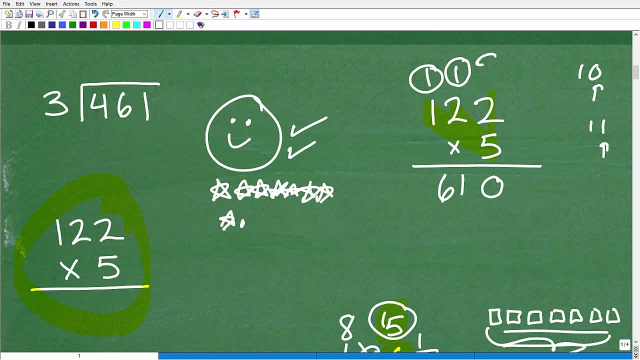 guys. right then, I must give you multiple stars and a Mohawk. Okay, Uh, yes, we did actually have Mohawks in the 1980s. I don't see them any, uh anymore, Uh, but maybe I don't get out enough. 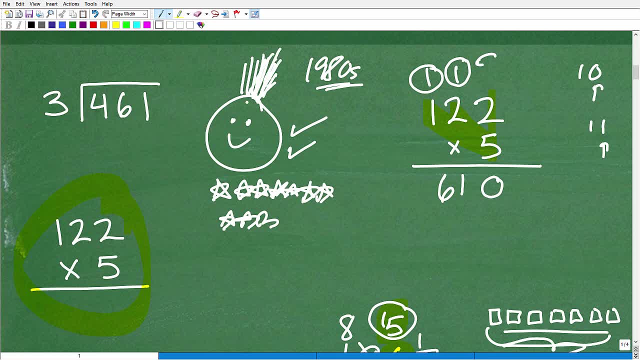 but uh uh, the bottom line is with: uh, you know, in the 1980s we used a lot of hairspray. Okay, It was probably quite dangerous back in those days with people's hair- a lot of hairspray. 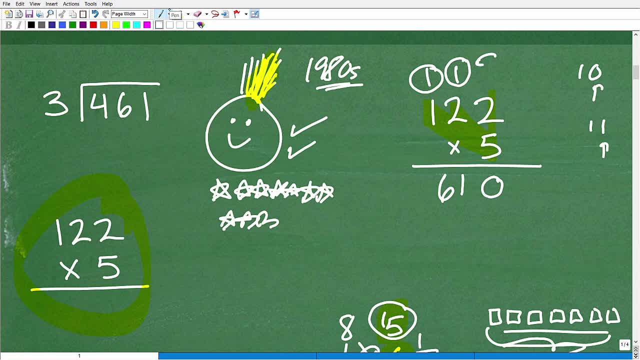 uh, probably wasn't good for the uh atmosphere as well. But the bottom line is, you know, we thought it was pretty cool and it's excellent and very cool If you got all three of these problems right, Uh, and you just like: yep. I remember I had great uh, uh elementary teachers. 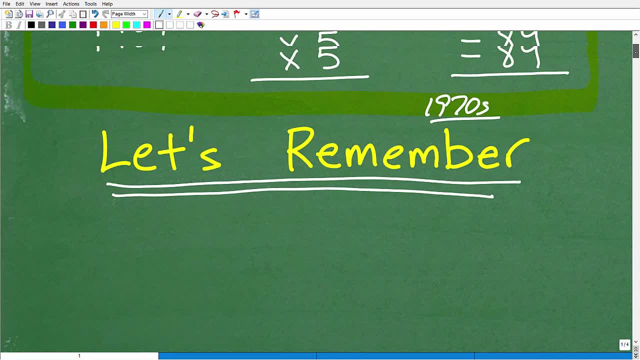 Listen, uh, no matter what, uh, you know teacher teachers you've had in life. you truly need to uh appreciate it. So I'm going to give you a five. Okay, So I'm going to give you a five. 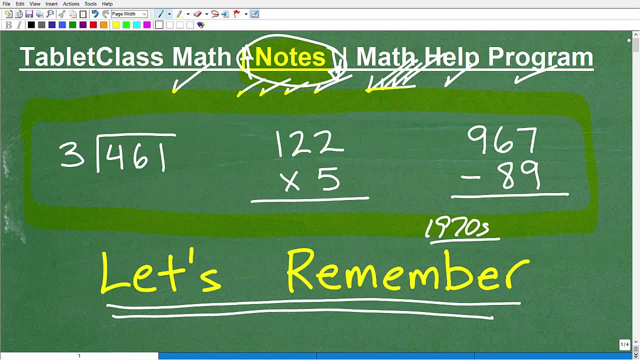 Appreciate them. Okay, Cause somebody taught you this stuff right, Like it just didn't just fall into your brain. Right, And you have. you have to really appreciate that. If you have these basic skills, then that's excellent, Even like my good old teacher way back in the good old 1970s. 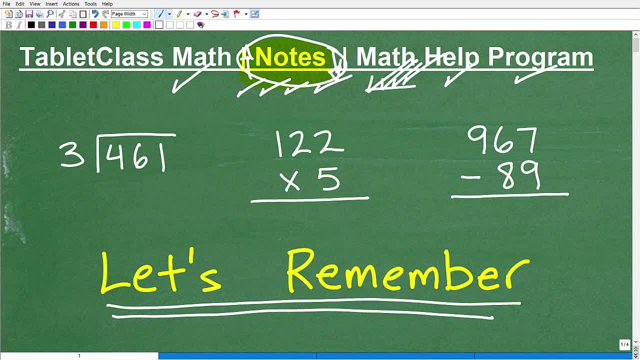 Um, I want to say her name was Ms Pete. Uh, I could be wrong, but I'm almost positive. Uh, I mean, listen, I think all my teachers, uh, you know, some of you might feel like I had bad- 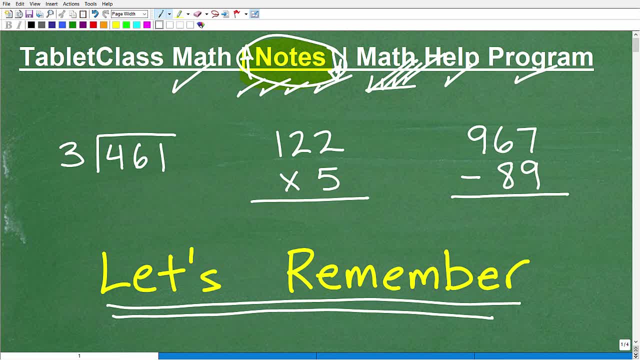 teachers. I had good teachers. Listen, anyone. I was trying to teach you something. try to have an appreciation, an appreciation for them. right, Teaching I can tell you right now from personal experience it's not an easy uh job whatsoever. right, It's very, very challenging. Okay, Um, 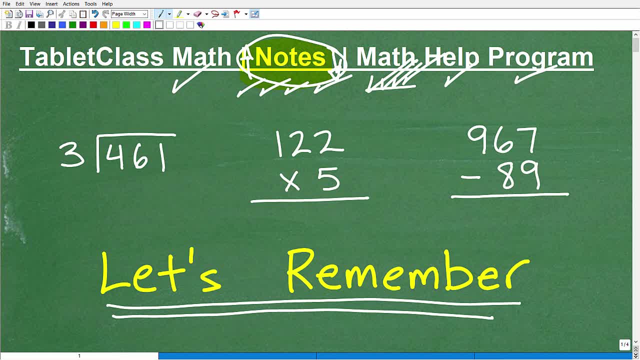 but there's a lot of- uh, personal rewards to it as well. So, anyways, what's the whole point of this video? Well, a couple of things. one, okay, Uh, freshen up on your arithmetic If you're a little bit rusty on it, because you're going to need it, especially if you're planning. 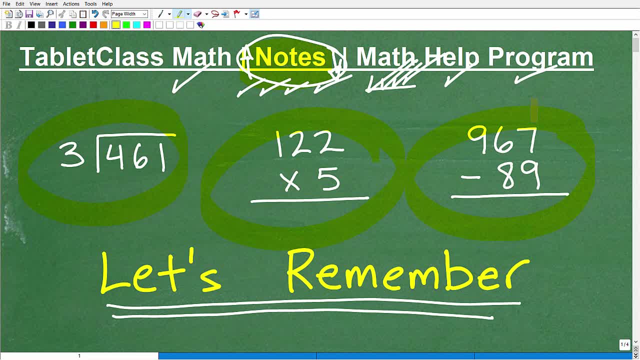 on learning math or taking more mathematics in your life. even if you're not going to, you know, if you're just watching this for the heck of it, you know still, you know, see what you can. uh, remember, because in practical application or practical terms, 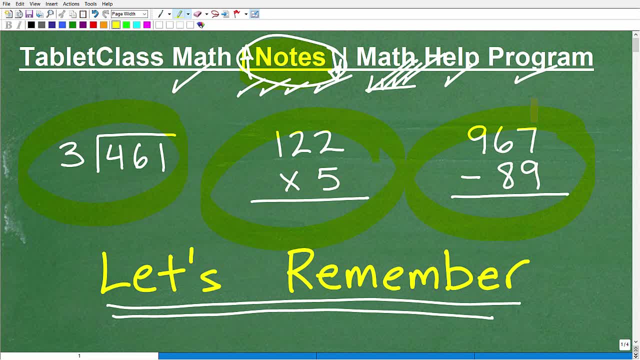 you know you still need arithmetic. It's very, very important, right? And the second point that I would want to make is that whoever taught you this and how they taught you that, you know, have an appreciation for them, for not only your math teachers, for anybody who's ever helped you. 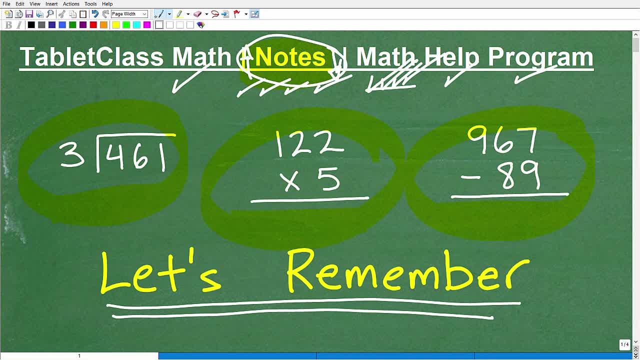 I think that's a good attitude that all of us can learn from, because, uh, gratitude is an excellent attitude. All right Now. with that being said, if in some small way you enjoy this video, please consider smashing that like button. that helps me out. And if you're new to my YouTube, 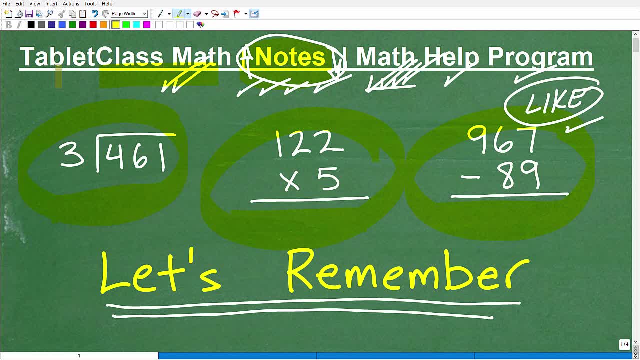 channel. please consider subscribing. I've been on YouTube for 10 plus years. I have over a thousand plus videos. If you'd like my teaching style, I have a lot of videos: basic to advanced mathematics, organized in various playlists. Okay, So please. 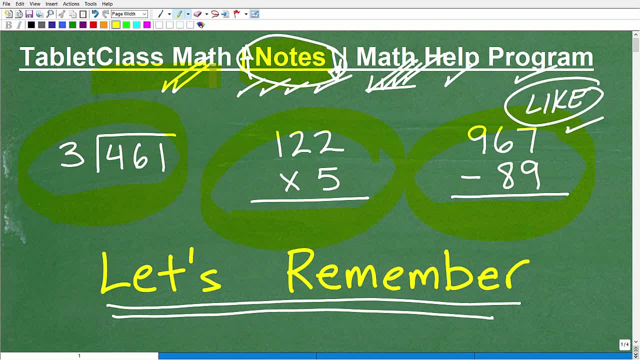 and I'm posting new content all the time. Uh, take advantage of that stuff, right? My mission is to try to teach math in a clear and understandable way. No one should be failing math. Okay, If you're doing your part, taking great notes, talking to your math teacher. 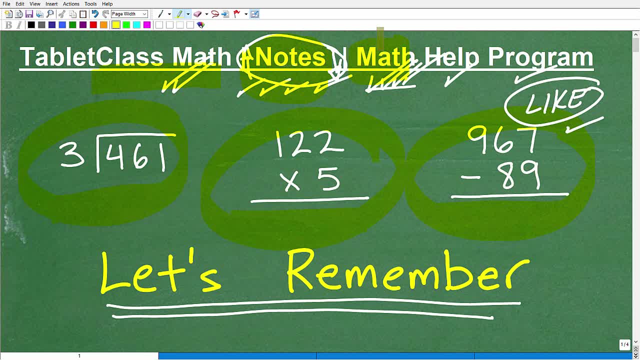 there's a ton of free resources out there that you can, you know, learn from. So, if you like my teaching style, you want me to teach you math? Hey, um, that's what I love to do. Um, you know. 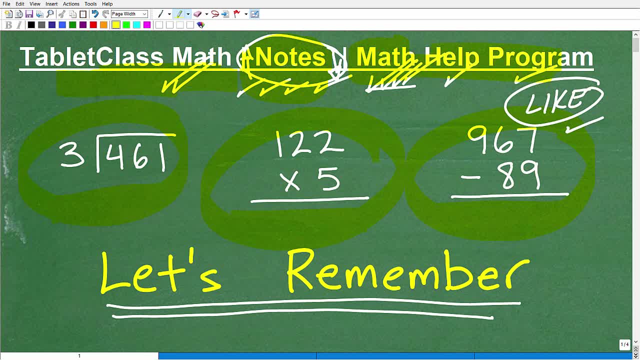 Hey, here, please watch my videos. Okay, But again, my best math help will be in my math help program- Tremendously comprehensive. So if you really do want to take it to the next level with my uh instruction, this is where you'll want to go. But uh, with that being said, I definitely wish you.